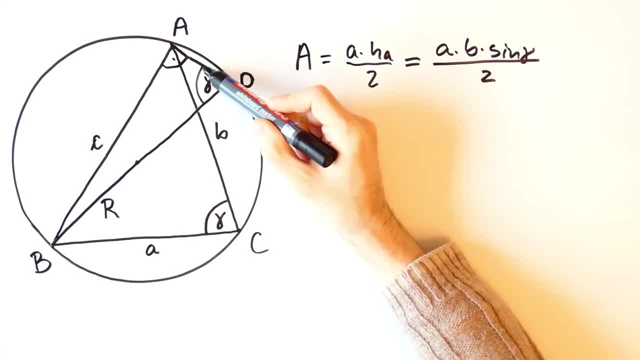 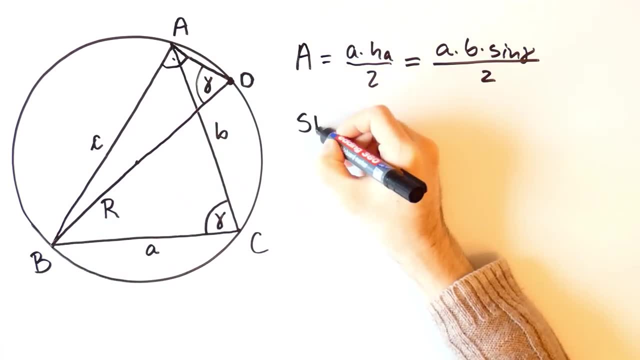 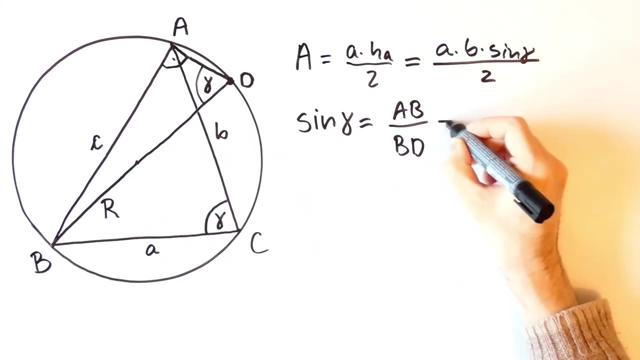 that the triangle ABD is a right triangle whose one angle is gamma. so the sine of gamma is equal to AB over BD, But AB is equal to C and BD is equal to 2 times the radius, since BD is a diameter. Now, when we put this instead of the sine of gamma in the expression for: 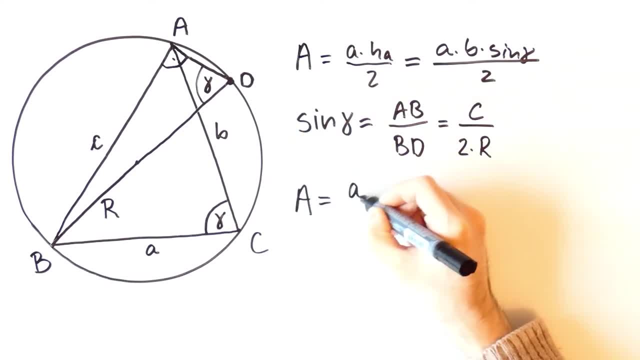 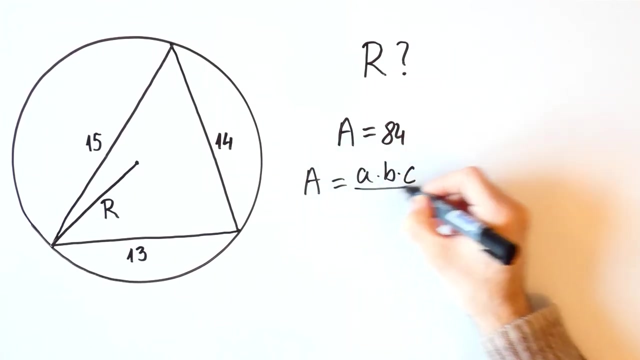 the area. we get that the area is equal to A times B times C over T. Let's now return to our problem. The area is equal to A times B times C over 4R, which means that the circum radius is equal to A times B times C over 4 times the. 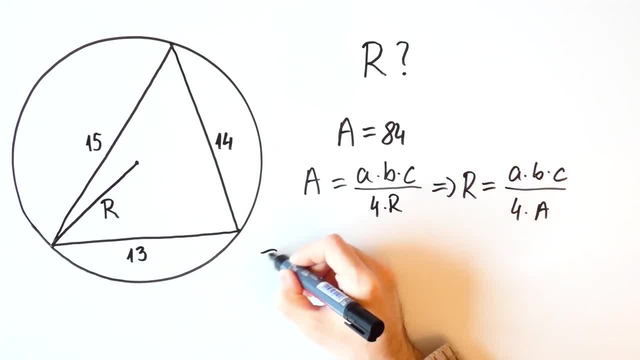 area And in our case that is equal to 13 times 14 times 15 over 4 times 84. But 15 is equal to 3 times 5 and 84 is equal to 2 times 3 times 14.. 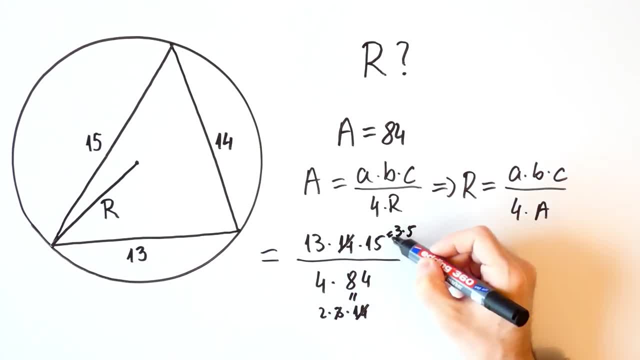 So 14 and 14 cancel out. 3 and 3 cancel out, which means that this is equal to 13 times 5 over 4 times 2, which is equal to 65 over 8, and that is equal to 8.125.. 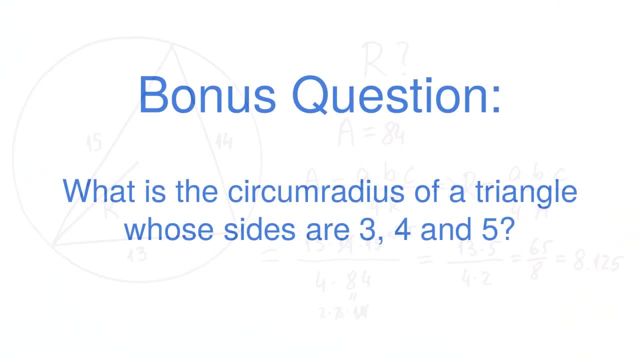 With that in mind, I leave you with this question: What is the circum radius of a triangle whose sides are 3,, 4 and 5?? That is all for this video. if you liked it, click the like button. it helps with the YouTube. algorithm And I'll see you next time. 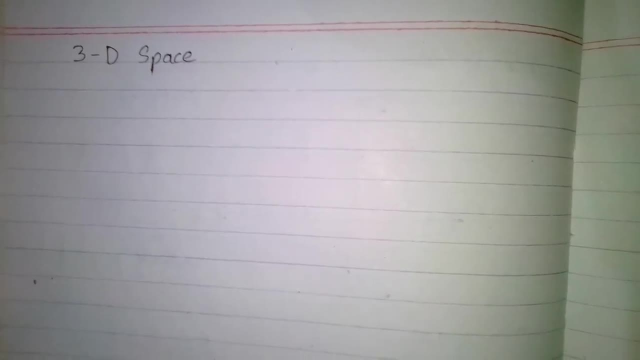 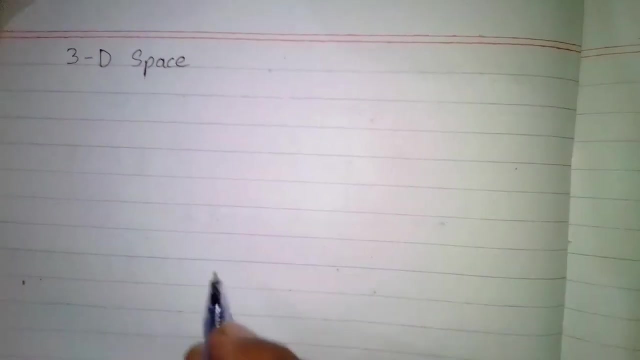 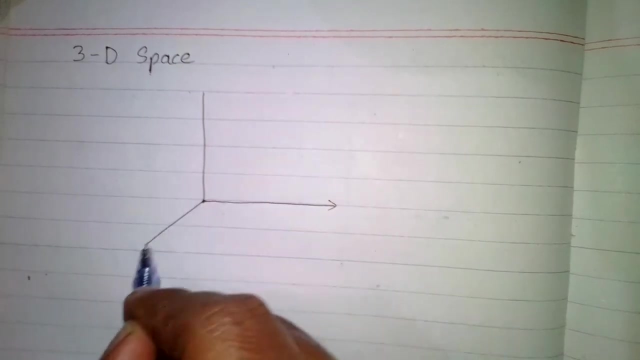 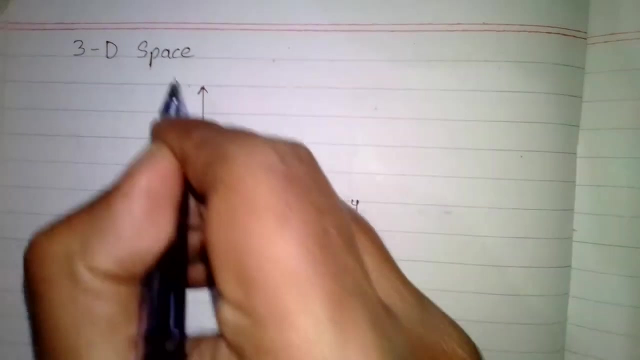 In this video we will discuss what is XY, YZ and ZX plane in three-dimensional space. So first of all, we will draw a three-dimensional space in which we have three dimensions: X, Y and Z- and they are mutually perpendicular.